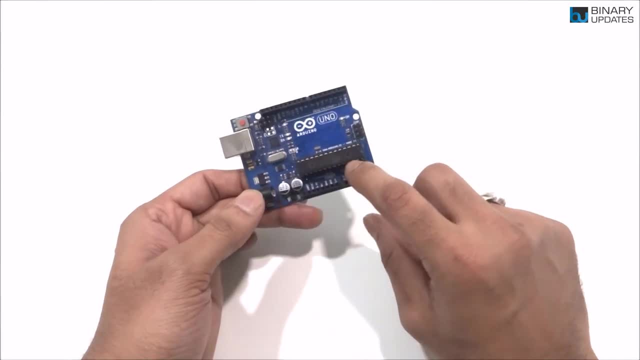 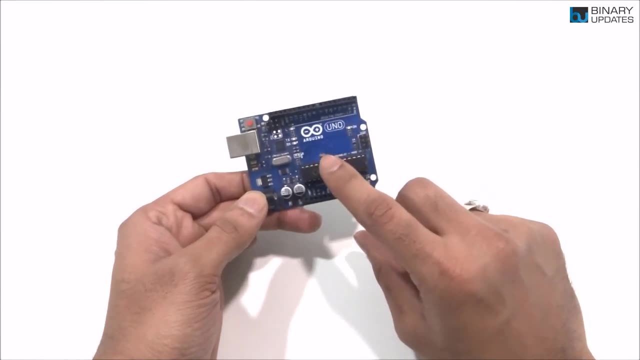 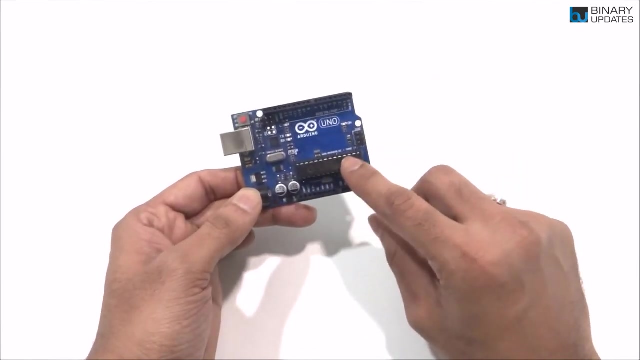 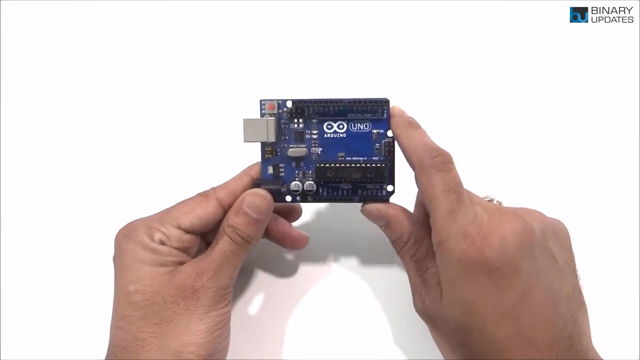 You can also check out our courses for Arduino and also for 80 mega 328. you can program this AVR chip- 80 mega 328 microcontroller- through the Arduino IDE using Arduino C programming language. if you are feeling like the normalcy is extremely tough for you in the beginning, before you go in and build the professional products, but later you can use the same board and you can scale it up to write a very professional embedded software for the same chip using 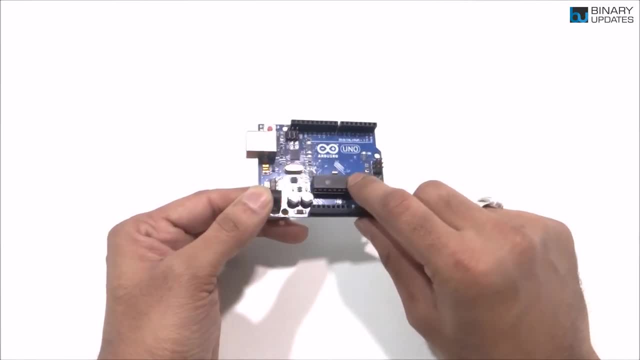 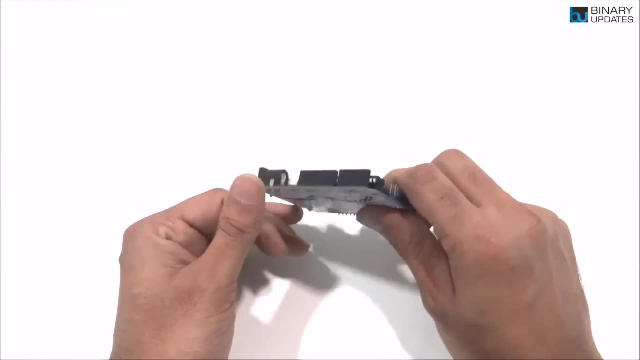 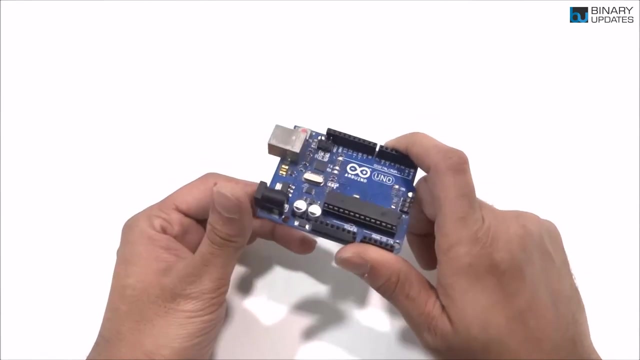 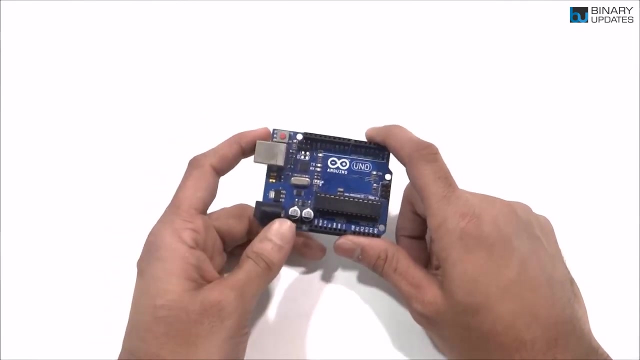 C programming right, and you can use the at the studio or microchip studio or something like this and write the bare C code and run and build a really professional product. so don't just understand Arduino as a little toy for the kids or something. no, you can really scale it up and I have seen really expensive products built around this 80 mega 328 microcontroller- and I'm not talking about just. I worked with a company in Germany and we were using it- AVR chips- to drive the pressure sensor. 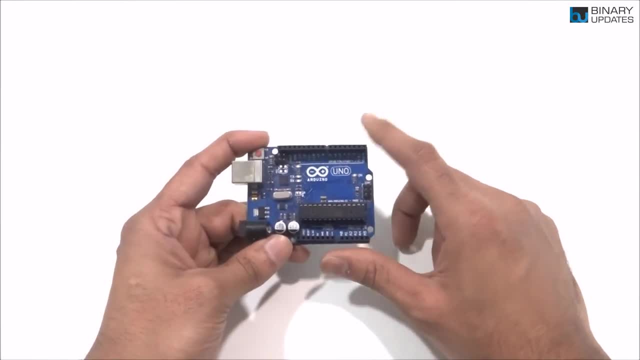 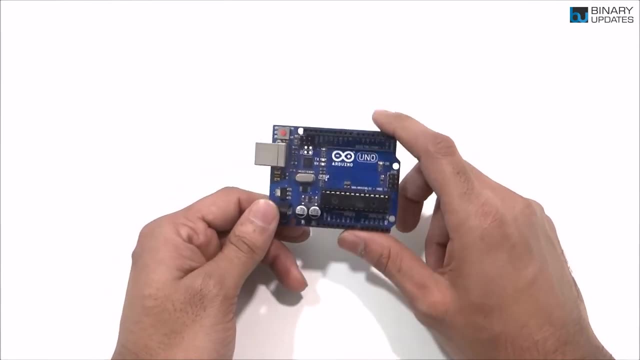 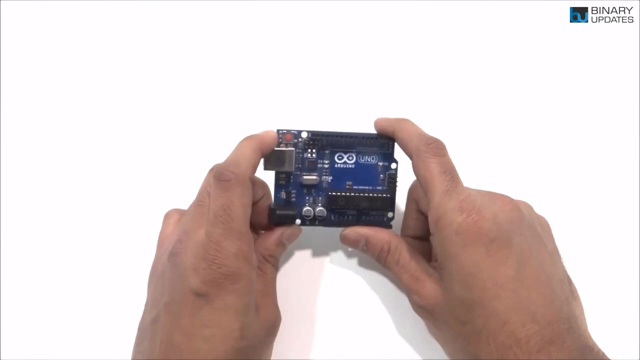 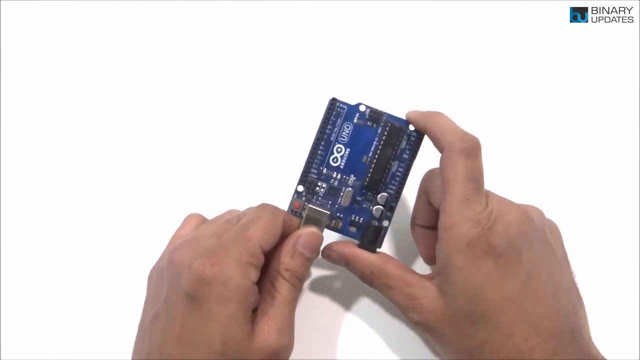 To measure the pressure in the blood vessels, right. so it's not really something like toys or something because you can read it and get it anywhere on the internet. it just doesn't doesn't mean that this is for the kids, it's really for the professionals. if you have the ability, if you have the right path, you can really use and scale it up this. so you, I recommend you to start with AVR 8 bit microcontroller, and the Arduino will be my first recommendation for you. 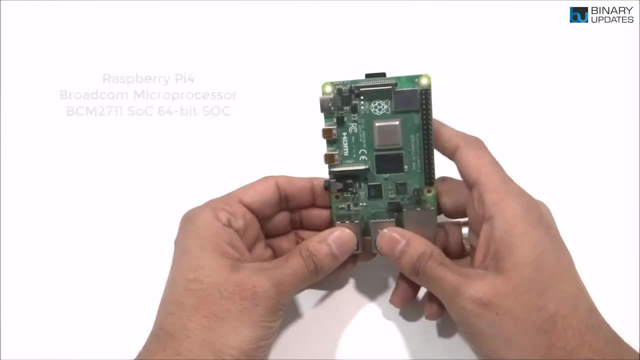 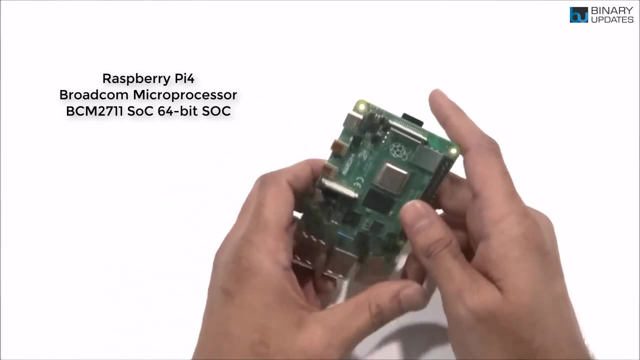 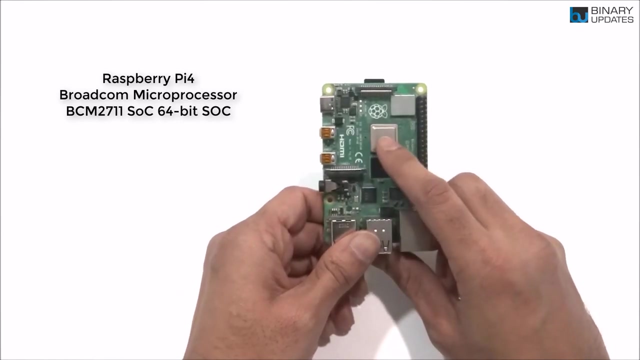 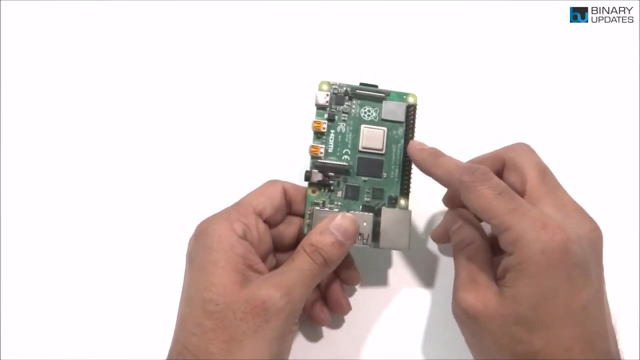 Now moving on to after microcontroller, I recommend people to start with the Raspberry Pi now Raspberry Pi 4 that you see in my hand. this is a microprocessor device. this Raspberry Pi has a chip, this microprocessor chip, which is CPU, from the Broadcom, and it has a 40 GPIO pins where you connect external sensors and actuators and all other things. it has everything. it has this: display connectors, camera connectors. 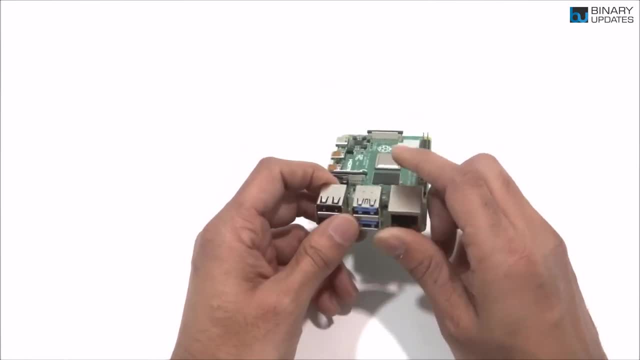 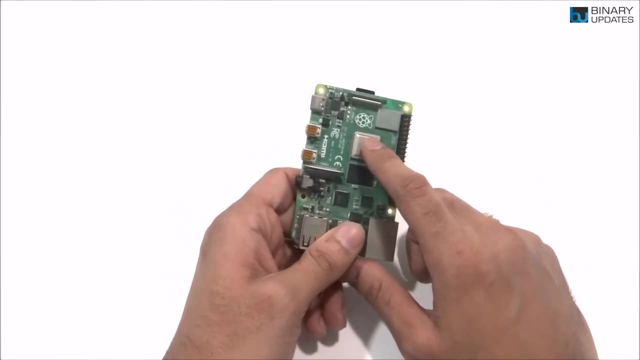 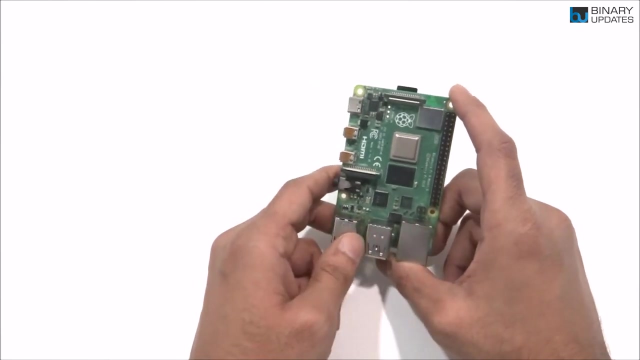 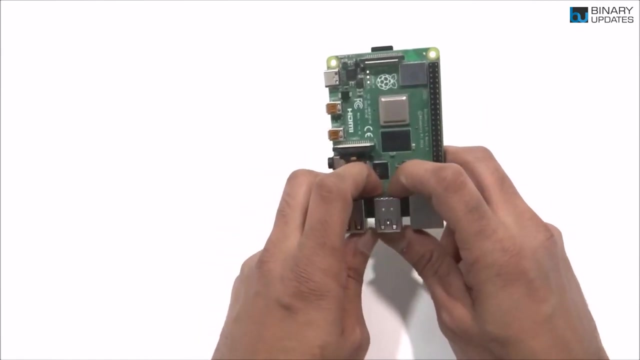 HDMI type C USB, 4 USB slots, Ethernet, Wi-Fi, Bluetooth- almost everything that normal computer has on the planet, and this is since it's a microprocessor. you have a great opportunity to learn the Linux as an operating system, because Raspberry Pi runs on Raspberry Pi operating system, Raspbian OS or Raspberry Pi OS, whatever you can call, because as an embedded system engineer, you must know when microcontroller and one microprocessor device and Arduino will be the best. 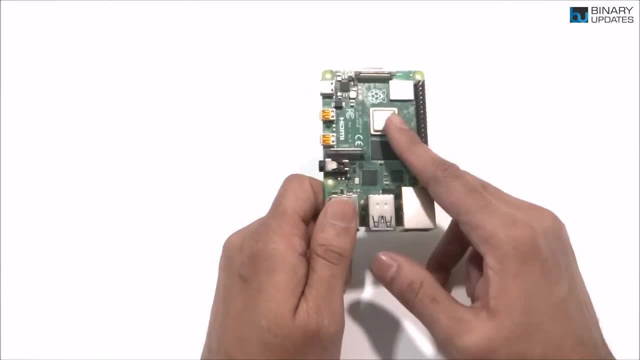 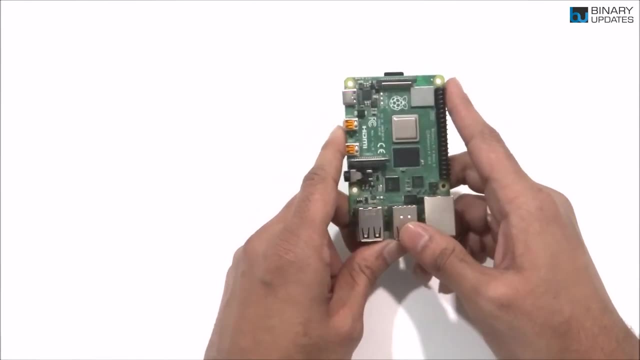 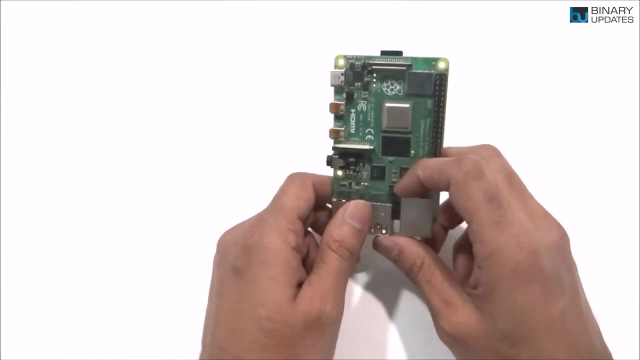 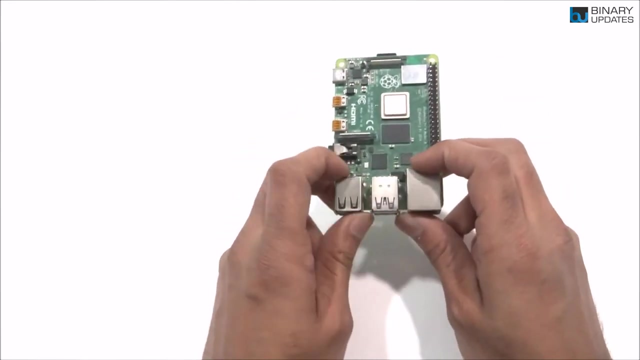 microcontroller to get start off and Raspberry Pi will be the best to start off the microprocessor. okay, CPU programming and all other stuff for the high level coding. so if you are building a product like IOT, Internet of Things or artificial intelligence to run open CV and camera image processing and stuff like that, really the Raspberry Pi is the way to go and I would not recommend other ones because, again, as like an Arduino, Raspberry have tons of online resources. you can also check out our courses. we 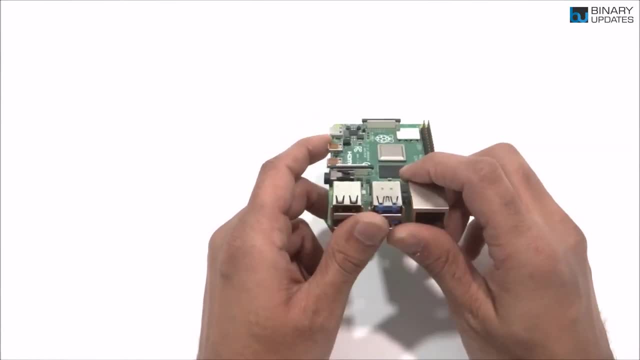 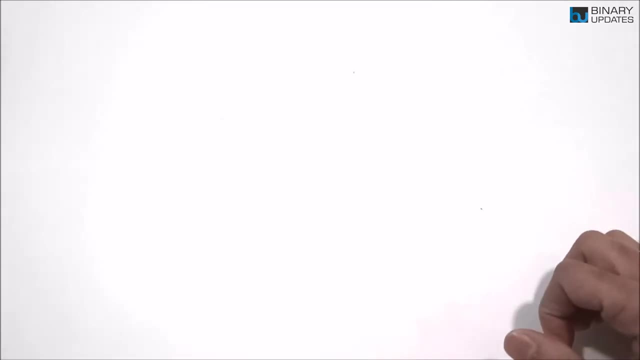 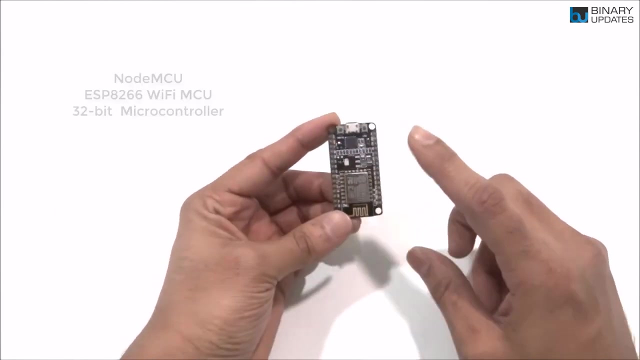 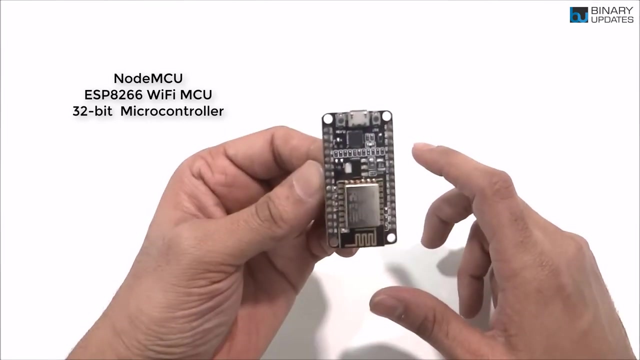 do have a very high quality courses to get you started with the premium class of support. so the second recommendation was the Raspberry Pi. now, once you, once you learn Arduino and Raspberry Pi with the microcontroller programming, I would suggest you to also get your hands dirty with ESP8266, which is also very popular with the name NodeMCU. you can see it- I don't know whether you can read, but it's really small, low cost. 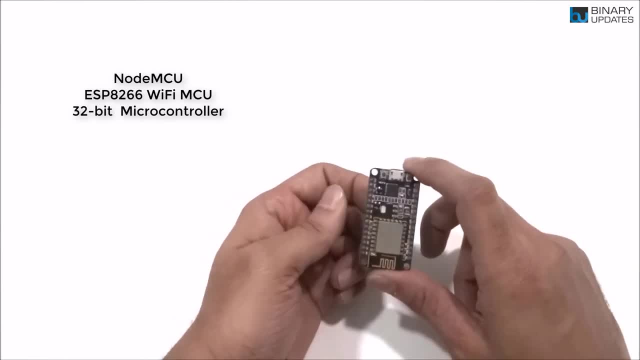 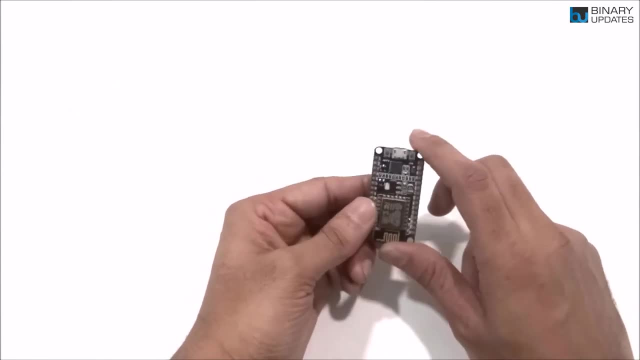 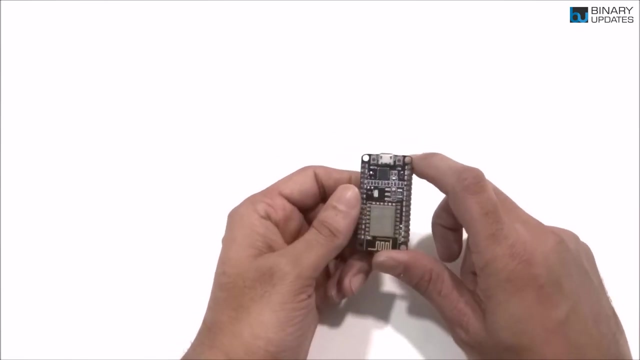 I think it's from the Chinese company called Espressif, and they made it a great job because, because this is a 32-bit microcontroller can be programmed through Arduino IDE or you can also program through the micro, Python or something, but I would recommend you to stay with C programming, Arduino C or the normal C. and the great thing about this chip is this has the Wi-Fi connectivity. so if you're building an embedded system project or embedded system product or solutions, and if you want to connect to the Internet, then I would suggest you to get your hands dirty with ESP8266, which is also very popular with the name NodeMCU. you can see it- I don't know whether you can read, but it's really small, low cost. 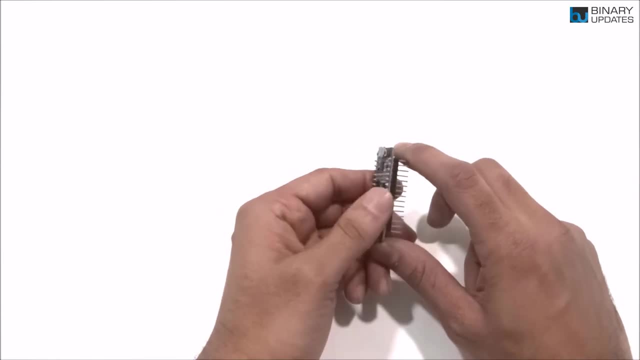 I think it's from the Chinese company called ESP8266, which is also very popular with the name NodeMCU. you can see it. I don't know whether you can read, but it's really small, low cost. this is easy to get start off and you can scale it up and it's really you can. 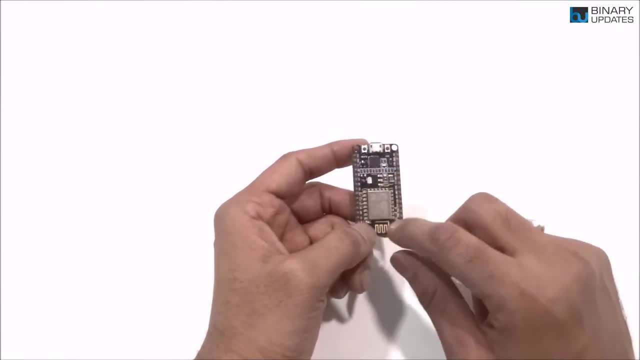 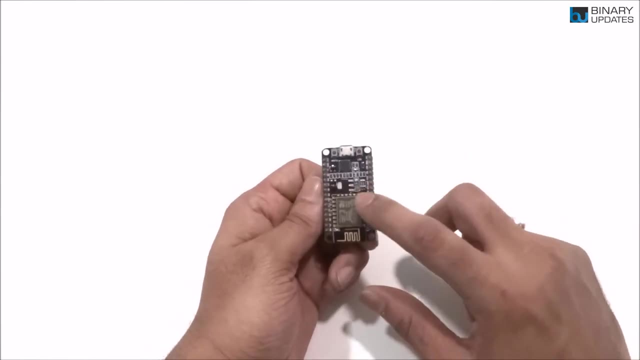 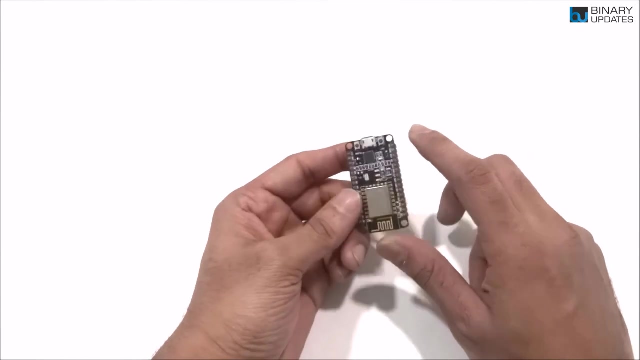 also go for production with this, basically because I have designed one commercial product around this ESP chip. so don't worry, I will. I will say it's a best to get start off, but for IOT it suits very good. the only problem this ESP means node MCU has is it has only one analog pin. okay, so you can only have. 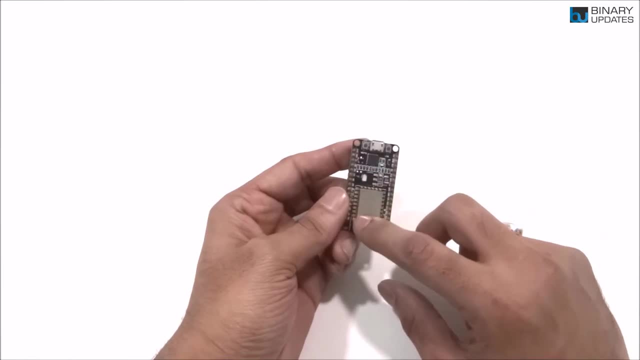 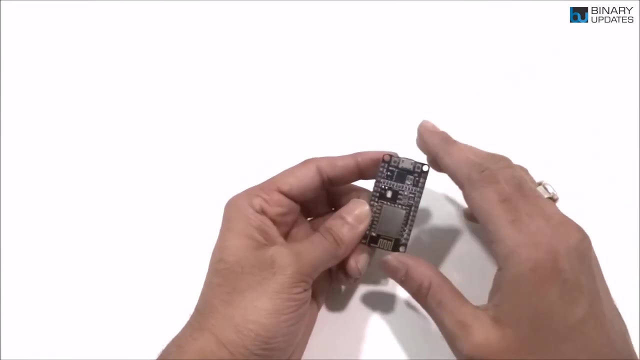 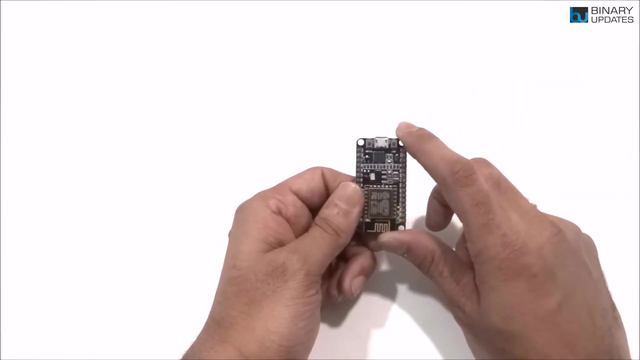 one analog sensor you can connect. but as far as we talk about the other interfaces, digital interfaces like serial UR I to C, spy communication and the other communication protocol, then it does support almost everything. so I would say this one goes to the third in my list of favorite microcontroller, or 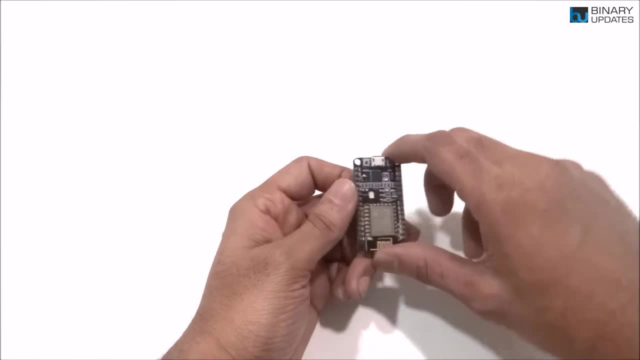 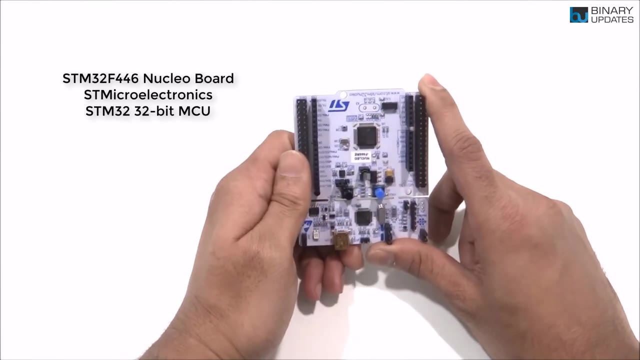 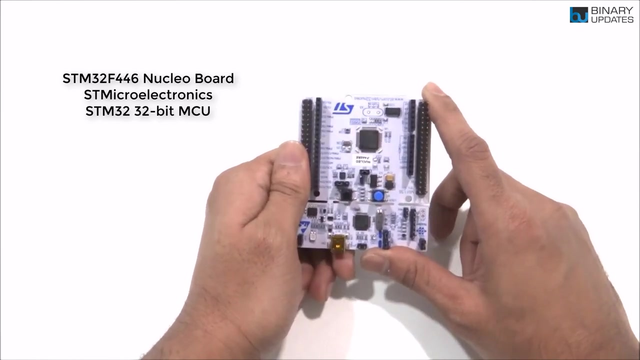 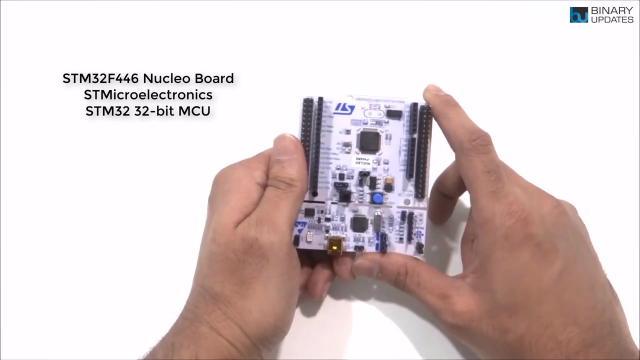 embedded system learning development boards. then the last one. I would suggest you to pick up this one. this is STM 32 and we all know STMicroelectronics is very, very, you know, popular name in the world of microcontrollers. they dominate basically. I seen a lot of products recently moving into the STM microcontroller and it. 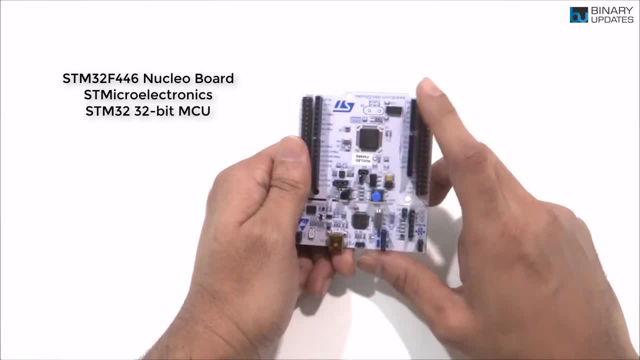 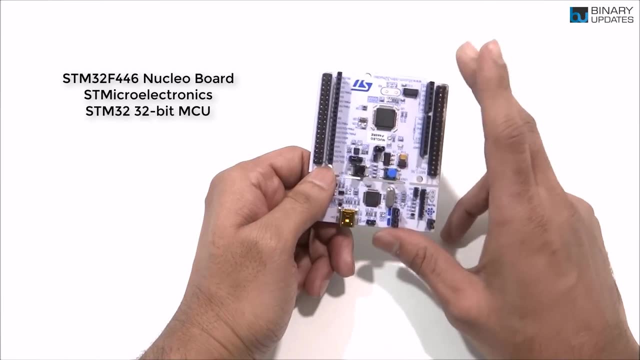 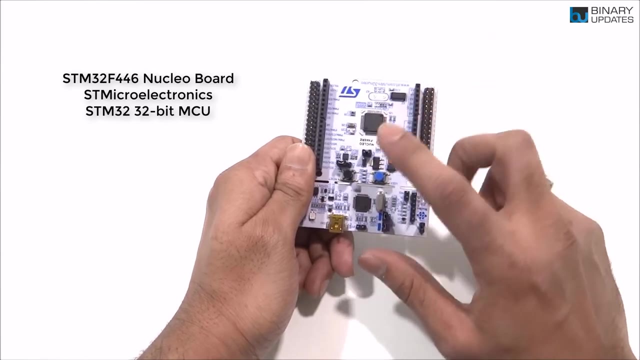 make a sense because they are cheaper. very powerful. not cheaper, I could say, but very, very powerful. this chip, and I would suggest you, even under the Nucleo there are so many, but I would suggest you to- to try and get your hands on with STM 32, Nucleo F446. 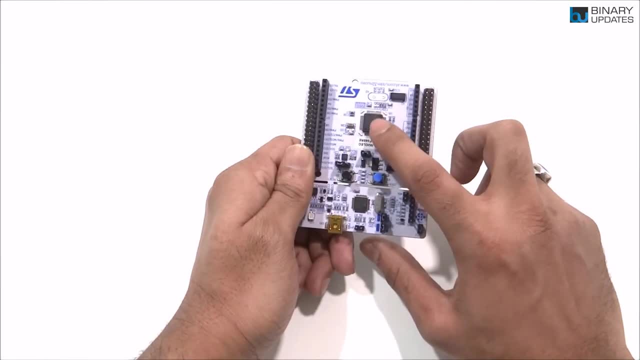 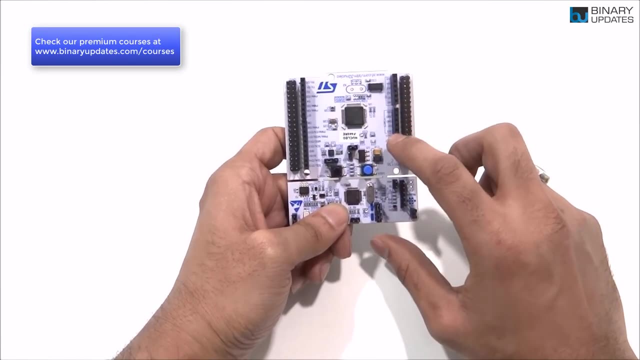 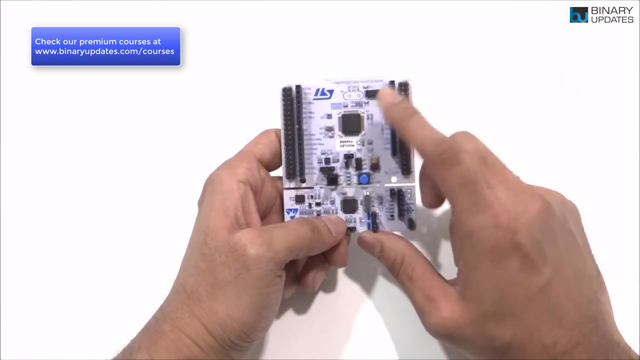 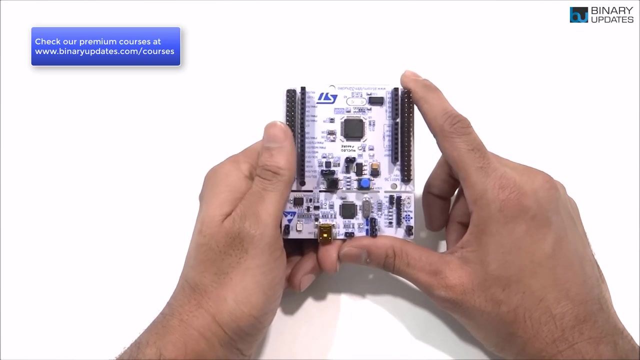 RE. so this is STM 32 F446RE chip and this board is very good because it follows the Arduino pin layout. so if you are moving from 8-bit Arduino to 32-bit STM 32 microcontroller, then you really don't need to buy so many additional components, because you might already have the Arduino shield. 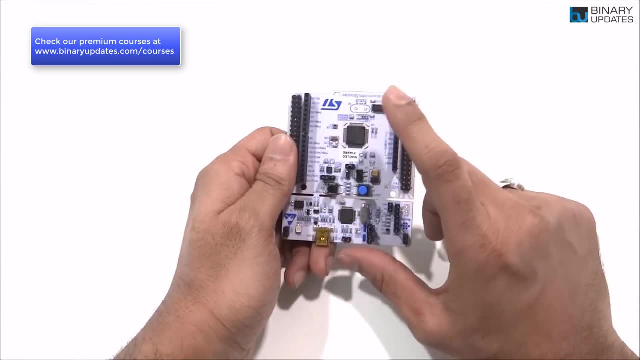 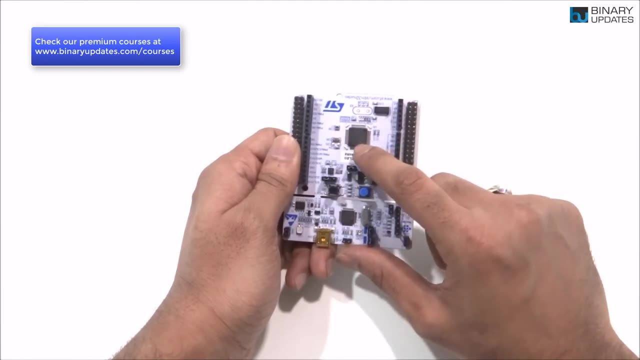 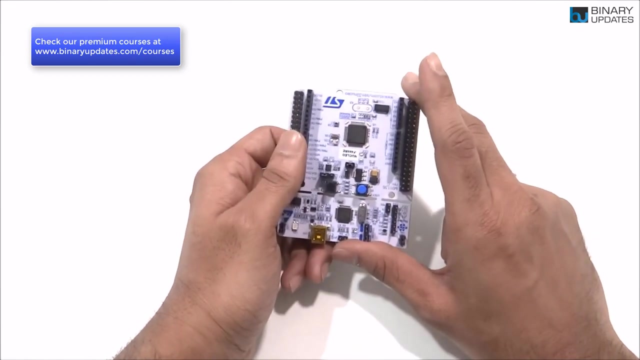 and connector and other things and you can stack it up onto the Nucleo board straight away and start writing the very, very complex applications embedded software for the STM 32 microcontroller and then build the project around this chip. this is extremely powerful chip. this follows 32. 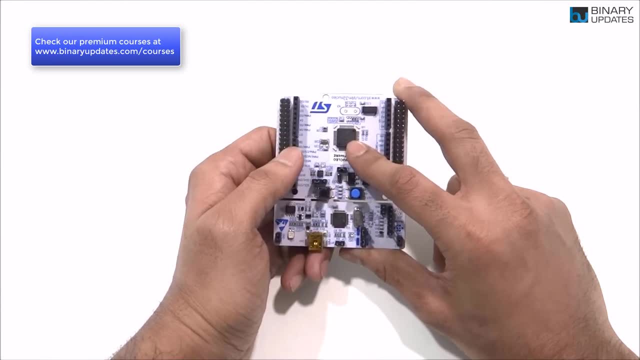 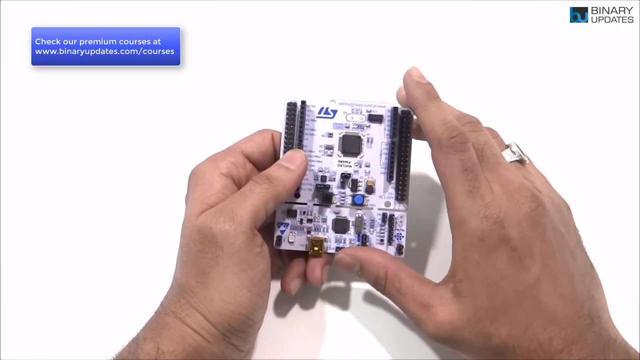 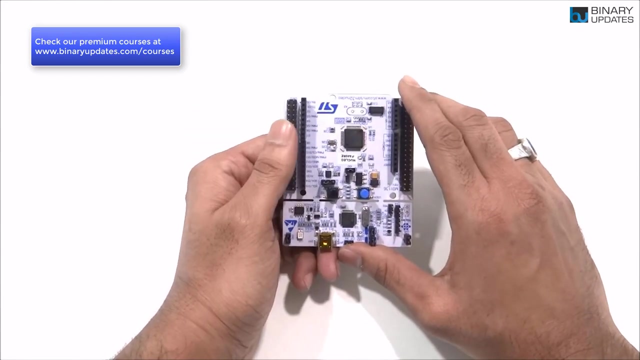 bit Cortex-M4 architecture and this chip can be clocked up to 180 megahertz or something like that and the clock is really deep to go. but this video is not really about clock, but this put into the fourth of my favorite embedded system learning hardware kit, and this is this. 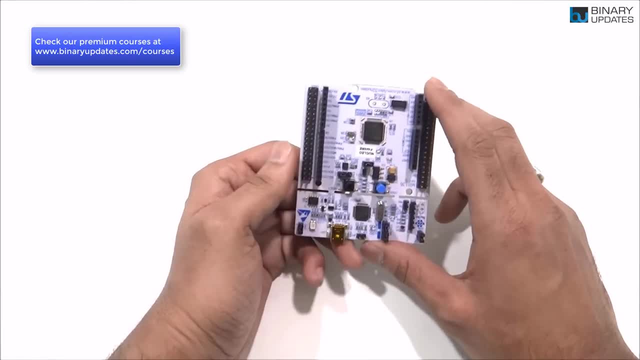 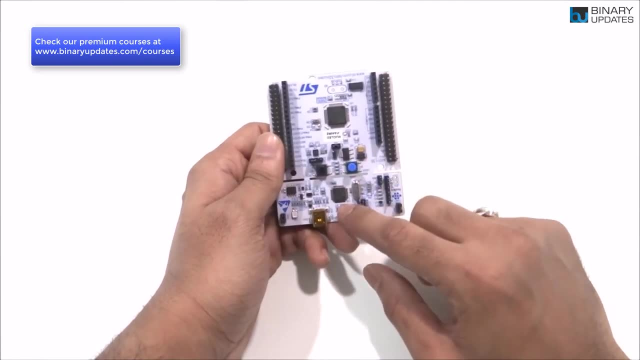 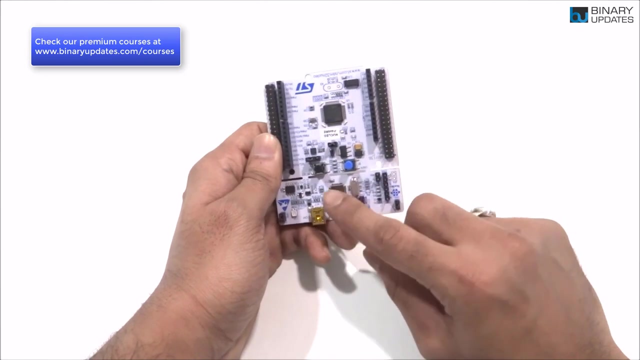 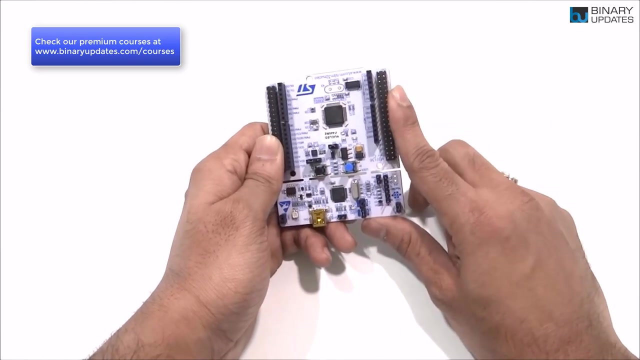 is really worth it because the one reason that I recommend to my clients for this chip to use or the board to use in order to learn this microcontroller programming because it has the onboard debugger. so the most of the micro controller board, professional microcontroller board- Has to buy the additional piece of hardware, That's the programmer and debugger fairing in the nuclear board. 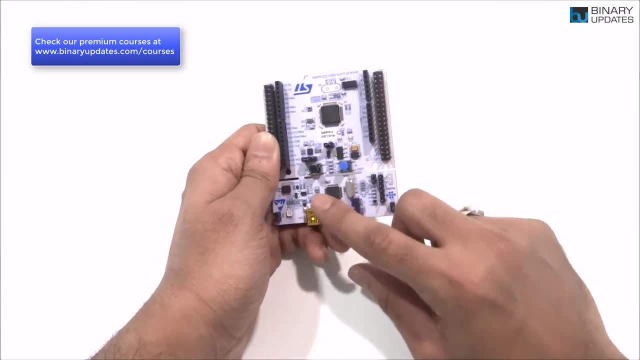 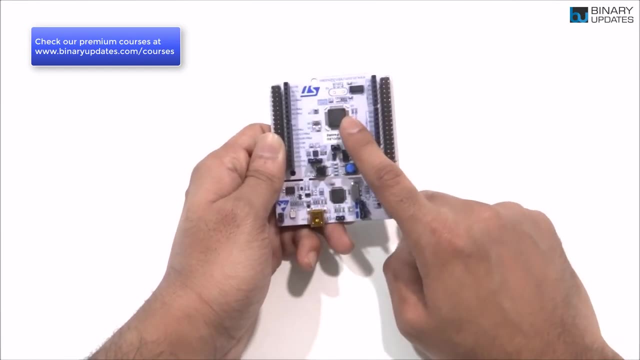 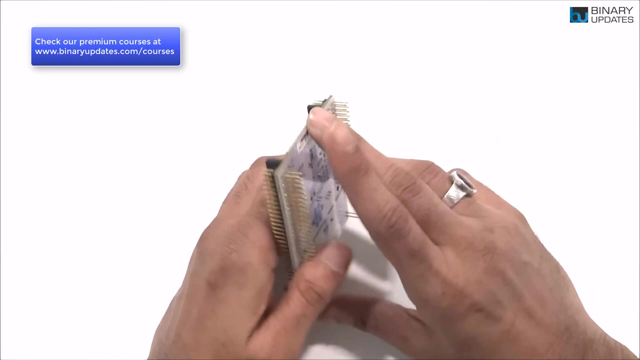 STM 32 f4 46 nuclear board. you have the onboard st-link debugger which makes it super simple to program this chip and debug the chip when you write an application- professional software- because The professional software will be very, very complex and you really want to scale it up and debug this application a lot. 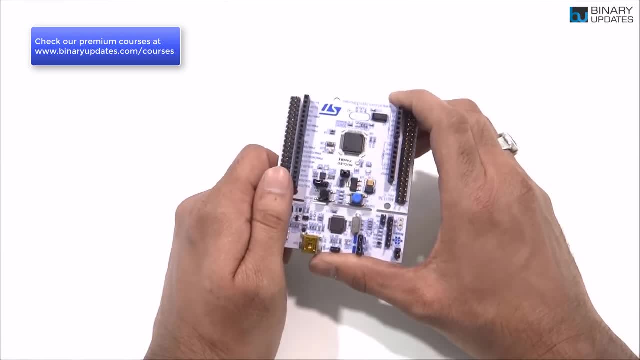 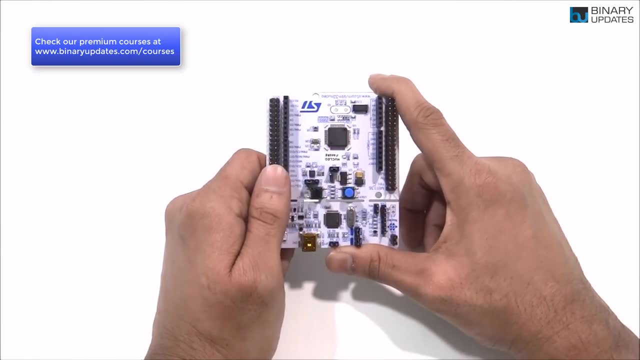 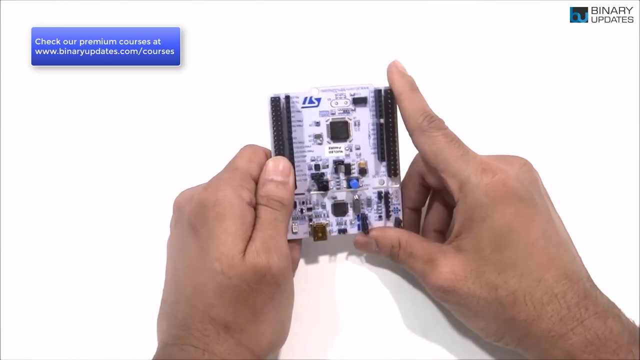 in order to fit into your expectations. and this is my fourth and The favorite hardware- you can really learn a lot like a DMA, I2C, I2S, UART and almost every protocol on the planet. you have this chip support. So when you are learning something and if you want to pick up the chip, not to 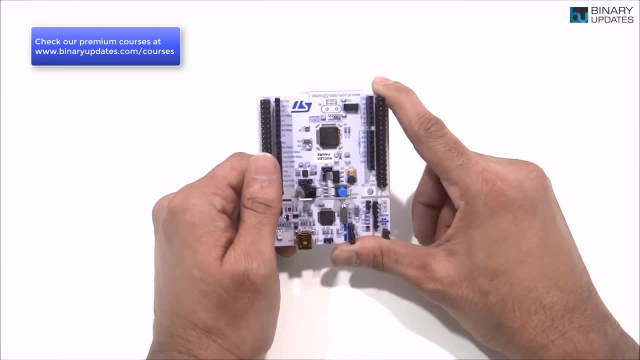 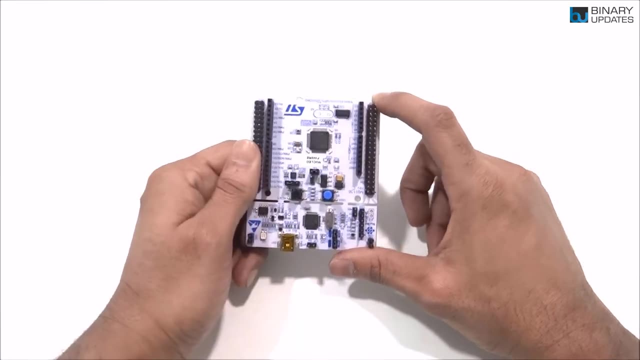 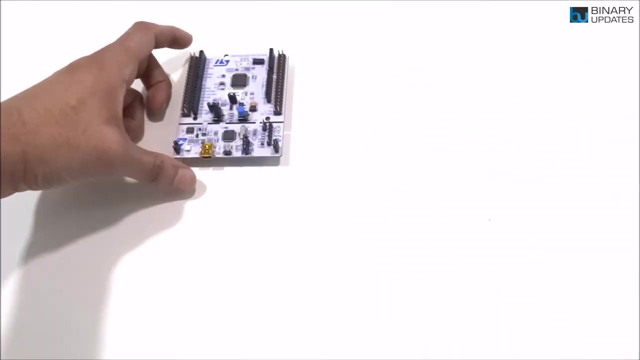 Move the chip from one chip to other chip when particular protocol doesn't support. To avoid this kind of nonsense, I think this is the one to go right. STM 32 f4 nuclear board. so this is all I have. like, this is my STM 32 f4 nuclear board and this is my. 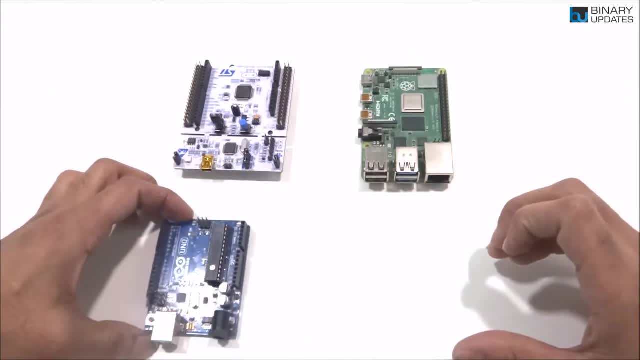 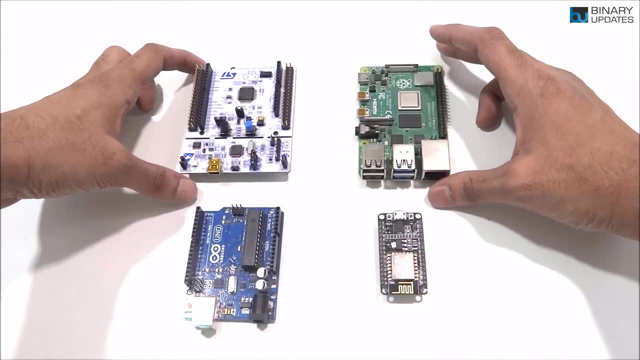 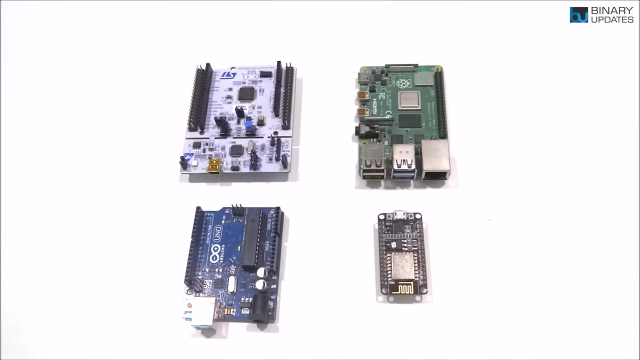 Raspberry Pi 4, then, as I said, I have this Arduino and then I have this Node MCU ESP8266. so these are my favorite embedded software learning kits or Controller development board, you can say, and I would recommend you to buy and learn about this now. 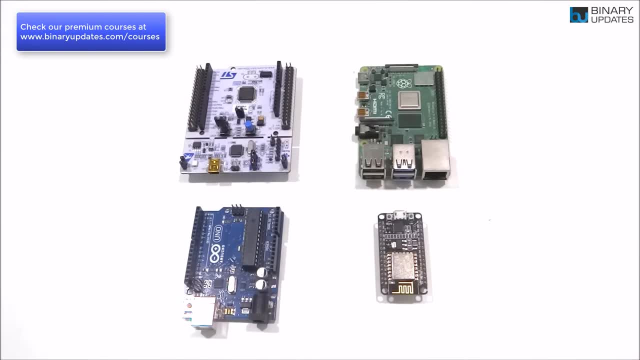 If you want to learn how to program these chips and write very professional Embedded software and really get a good job- high quality, high paid job- Then check out the link in the video description. And if you have any specific question about learning embedded software and embedded hardware or anything to do with embedded systems,